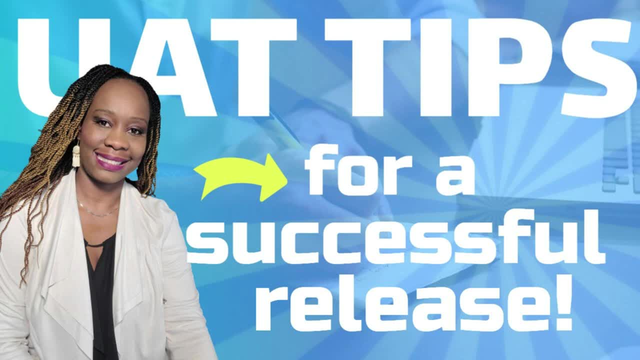 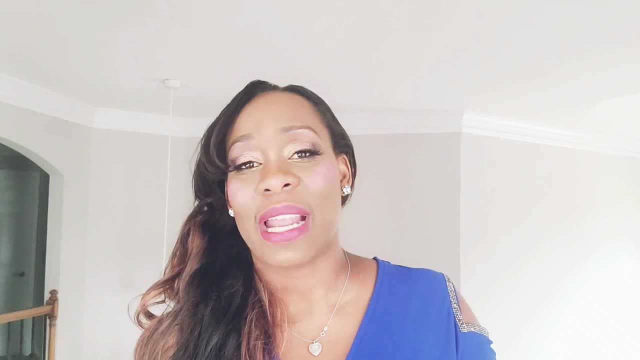 telling you how to do the UAT, what you need, the environment, all that stuff, But I realized that you still need some more information, right? Some of y'all are really struggling to get this thing done, and I want to help you the best I can. So in this video we're going to talk about 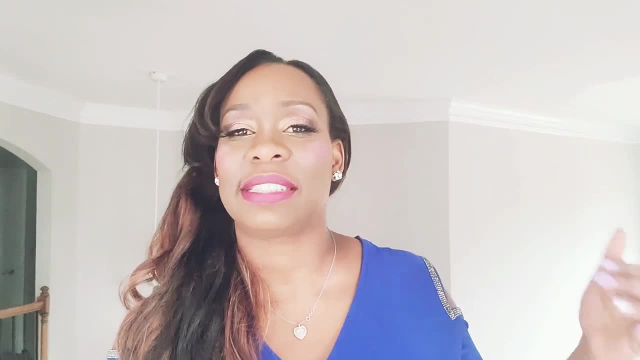 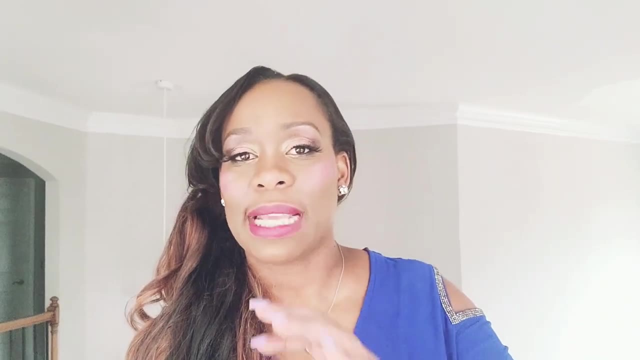 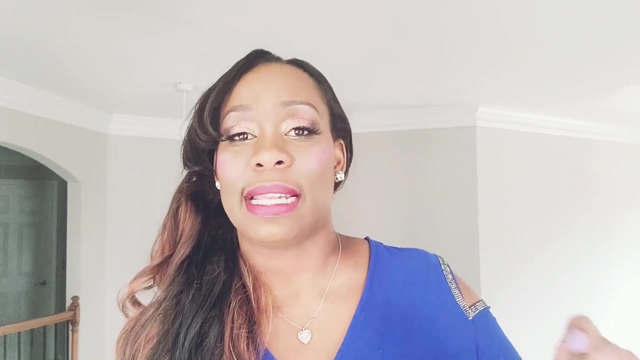 what is the process that you need to have to have a successful UAT test, What steps should you be taking, What steps should you avoid? And walk you through, step by step by step, how you should be doing the UAT. So I'm going to walk you through the process: steps, what starts and then. 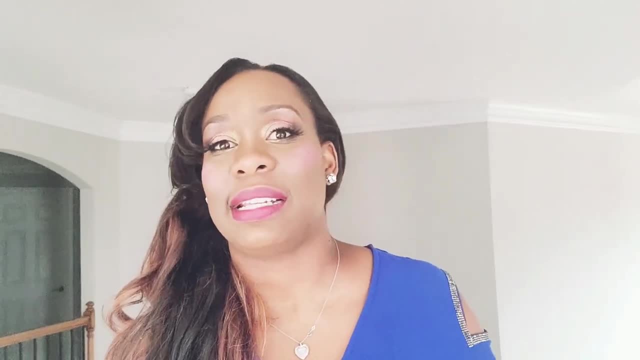 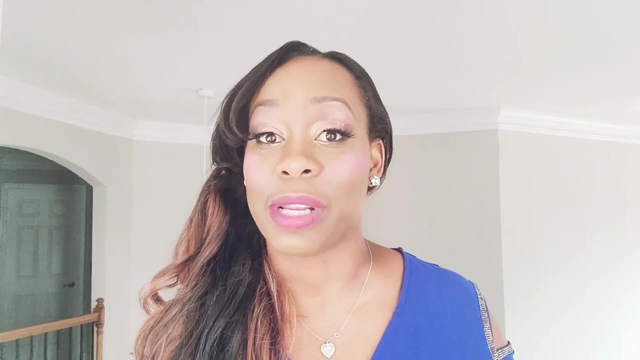 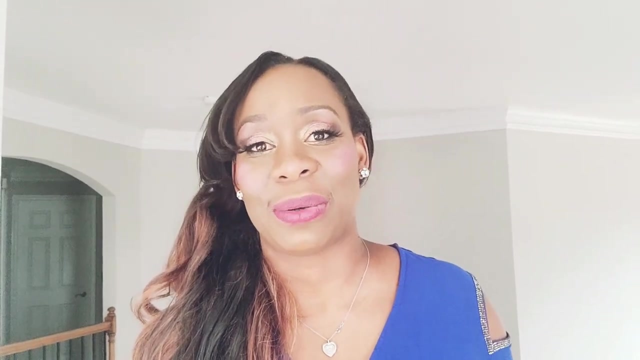 next and then what happens next and how do you manage all the bugs and what's the best thing to do for recording the bugs, things like that. I'm going to walk you through that with what a real world project is doing And then give you my suggestions as to what you should be doing and the pitfalls to avoid. 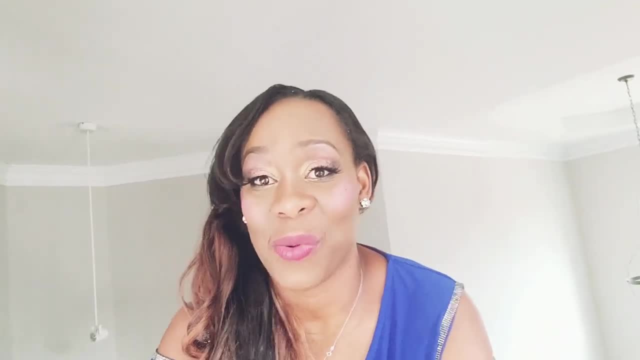 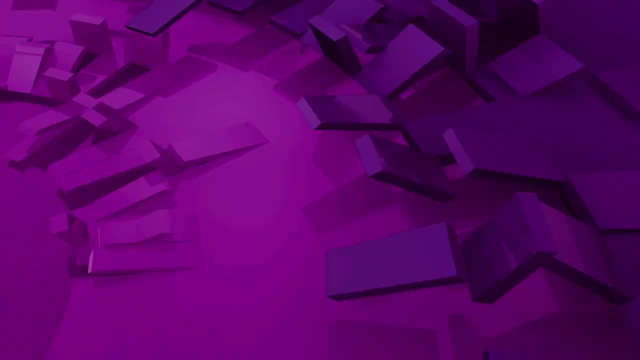 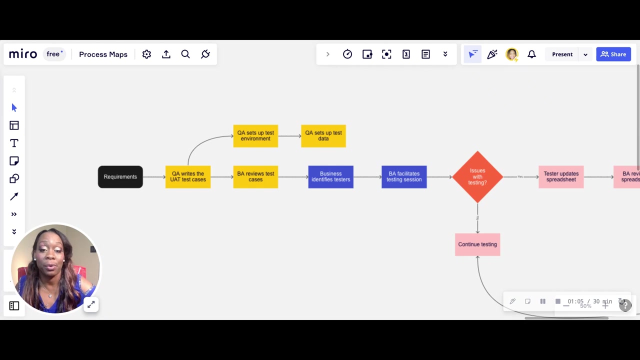 All right, so that's going to be our video today. I hope you enjoy it And let's go to my office where we'll work on it together. See you there. All right, everyone. So here we are in my office and we're going to be walking through. 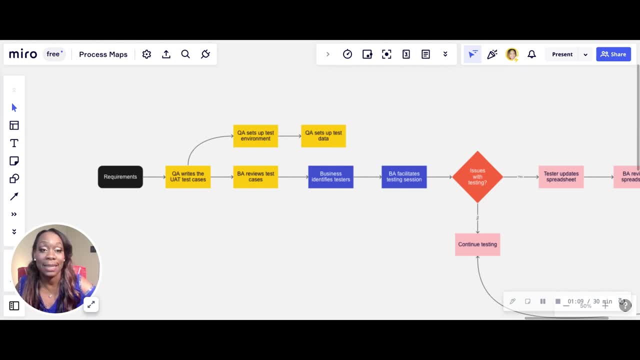 what you're looking at right now, which is a process flow for a UAT process. I'm going to walk you through the as is, step by step process. This is what they're doing on a real world project today, And I'm going to give you some. 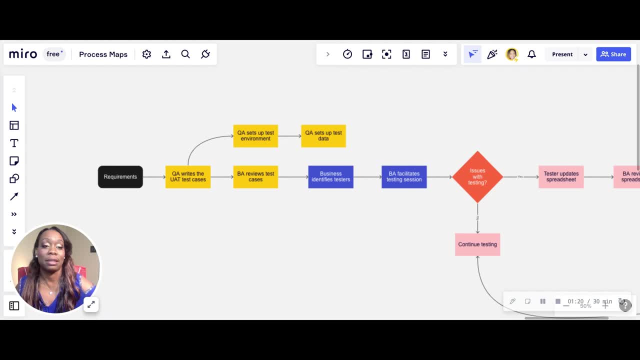 pointers as to what we should be looking out for and not do. So some of the things here we're going to keep, some things are going to throw away because we can do it better. So we start off always with the requirements. Let me zoom in a little bit, Make sure you guys can see it. 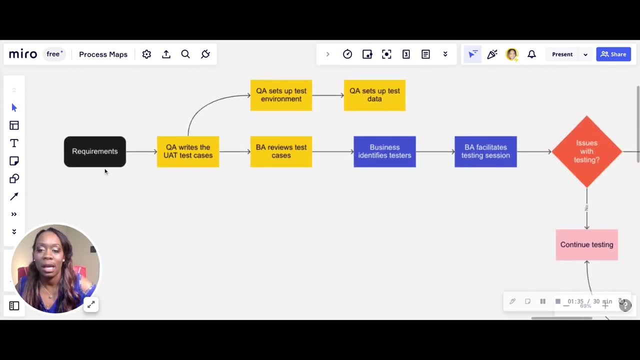 There we go. Okay, I'm using a tool here called Mirrorboard. If you've not used Mirrorboard before, it's pretty good for you to do flow charts or do a collaboration session Or a workshop, virtually ideation session- all of that. It's a very good whiteboarding tool. 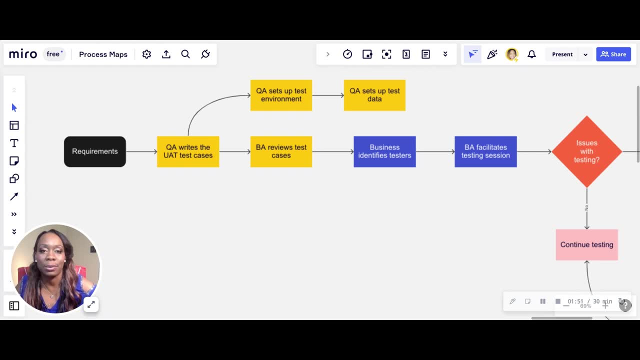 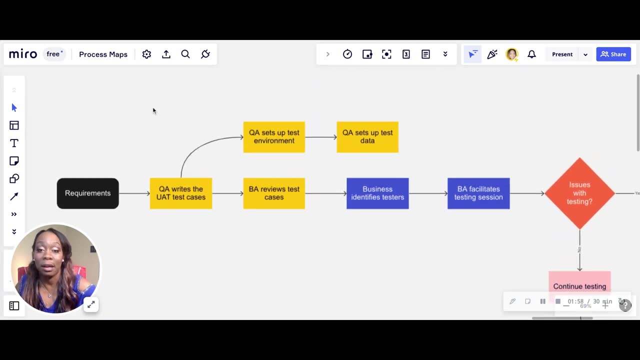 You can build all these different types of things in it. So I think this is a great tool for you to be exposed to, if you've not used it yet. So you start off your requirements. You start off your process by understanding the requirements. right, That's the very first thing. If you have not, 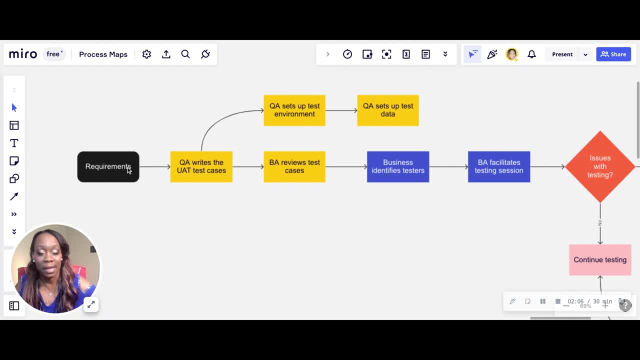 written the requirements up to this point. you have to be very familiar with them because you have to know what you're going to test. Then, in this process that they're doing today, the QA was writing the UAT test cases. So the QA was writing the test cases And the QA was also. 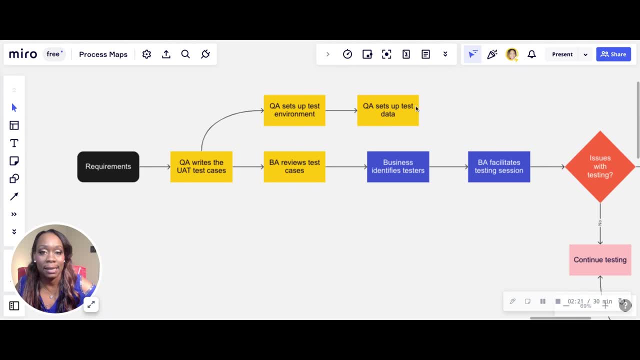 setting up the test environment and getting all the data that they need, the access rights, the data sets that they need. make sure they have everything they need to be able to perform the test. All of that was being done by the QA And then they would hand off to the BA And the BA. 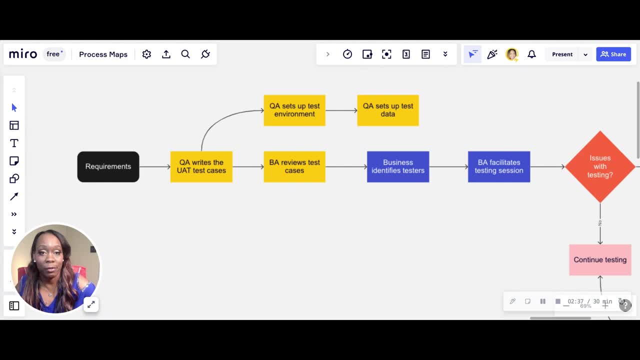 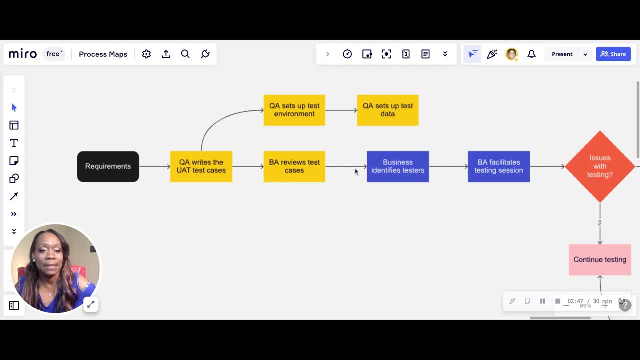 hand off to the QA, And then they would hand off to the QA, And then the business unit then would identify who are the people with the right knowledge that could help to do this test, And so the business unit would go identify the testers, And then the BA would facilitate the testing. 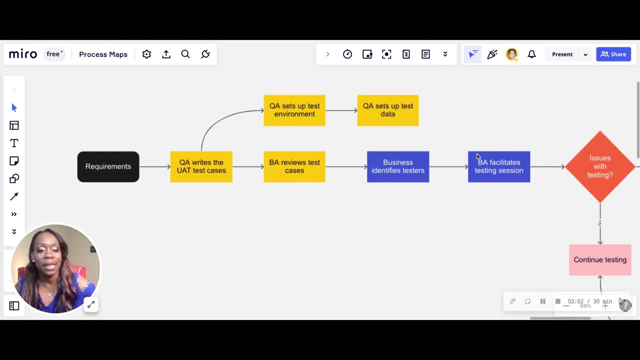 exercise, So they would set up the calendar meeting, And the way they were planning on doing this testing exercise was: it's a huge project with a lot of different moving parts and many, many different teams, So, because it's hard to coordinate people, what the plan was was that they'll give each person two hours that they have. 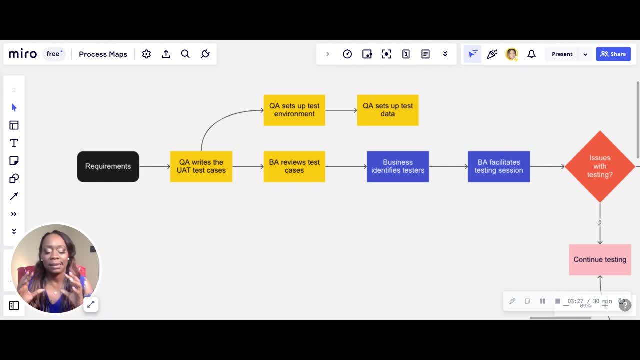 to dedicate to testing per week. But I think they had said they would give each person two hours and the person can choose which two hours is most convenient to them. So one person could choose nine to 11,. one person can choose one to three, et cetera, et cetera. right, So each person would 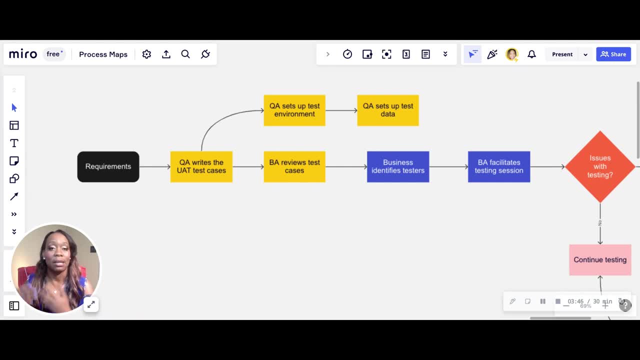 be going in on their own looking at the test cases and conducting the test, And that's how they would do the test. So, in an effort to be, they know that this is not the person's real job. Their job is to do. 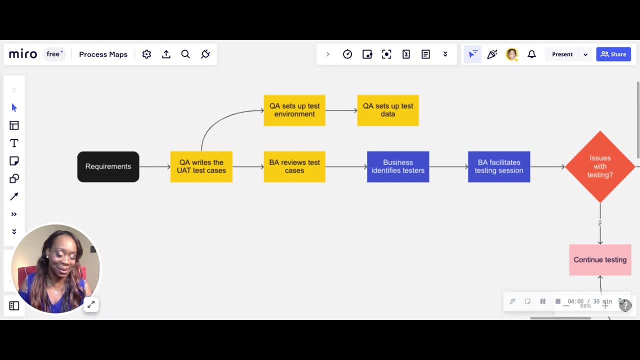 something else. We're just taking them off of their job for a minute or two hours and having them apply their skills to the testing effort. So they didn't want to disrupt everything too much. They wanted to give them some freedom. So that's how they planned to do the testing. So that's how 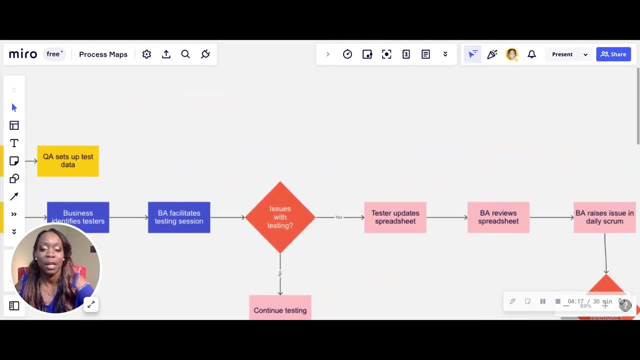 the sessions was being done. I have some comments on that Now, in while they're doing the testing, while they're doing this test, if they find a bug or they find an issue, what they would do is they had a spreadsheet and the instruction would be that the testers would go on the spreadsheet and 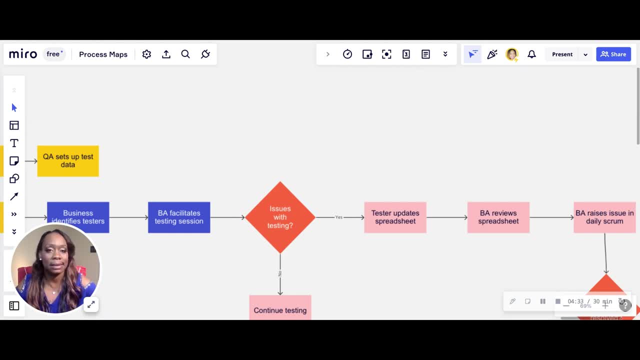 log the bug to say this is a test scenario. I was testing. This is a bug I found, put a screenshot on there And that's how they would log what the issue is. Now they plan on having multiple spreadsheets for each tester And the tester would just take a couple of spreadsheets and fill in. 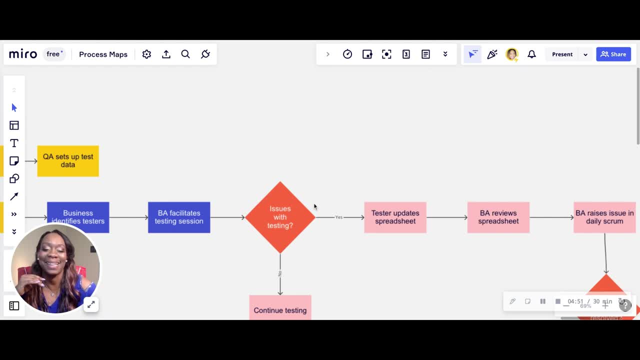 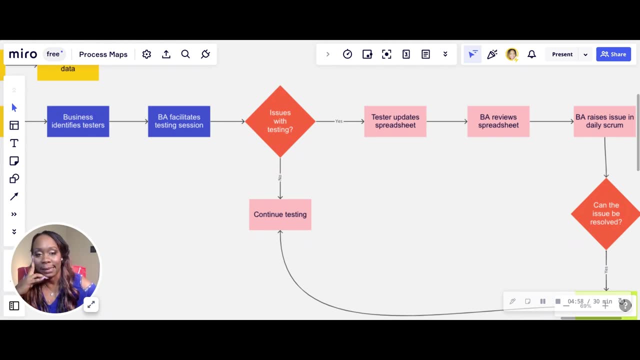 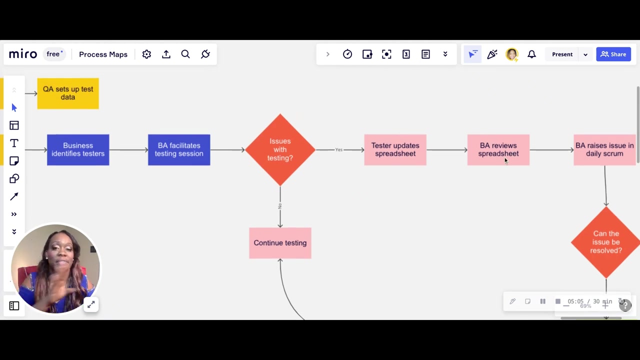 the bug they found. I have comments on that too, but I'll tell you later. Now, if they haven't found any bugs, then they would just continue with the testing. Now, when they find the bug, the BA would review the spreadsheets. So they'll look at the spreadsheets for each of the testers and see what. 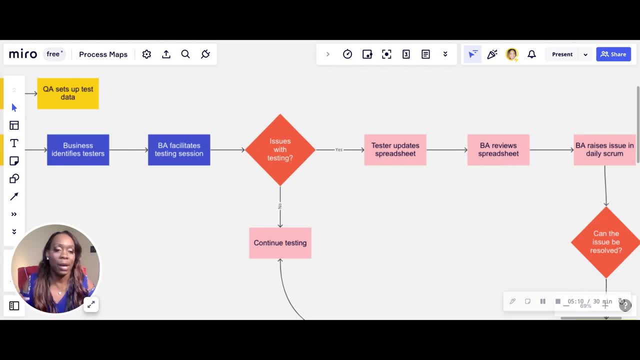 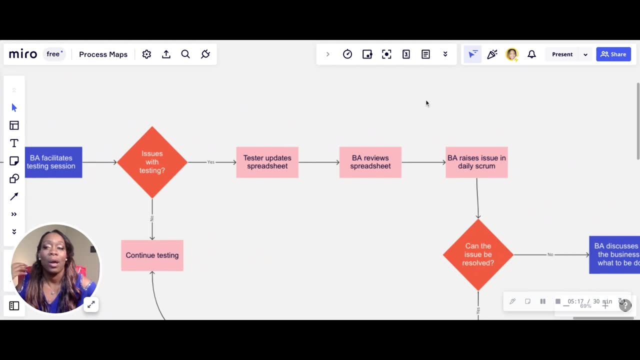 bugs they have logged And then, based on those bugs, the BA would go to the daily scrum or the standup and would raise those bugs in the daily scrum to say to the team: Hey, we have found these bugs in UAT. We need to have these resolved. Now they were doing what we call. 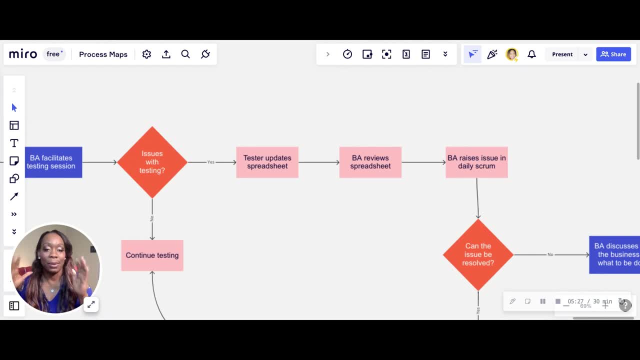 a regression sprint, which is this is going to be the sprint that we've dedicated to fixing UAT bugs. So whatever comes out of the UAT would be the most important thing to work on for the team for that sprint, so that they can get the UAT bugs fixed so that they can retest. So when the BA raises these, 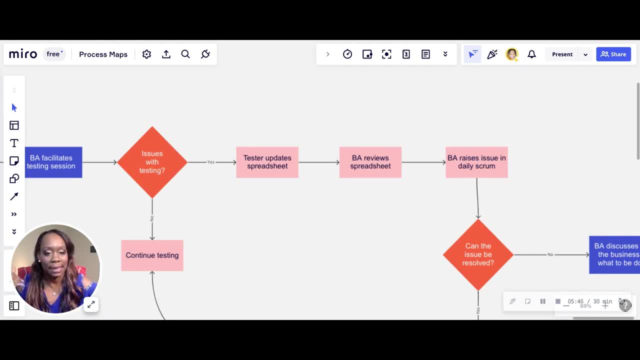 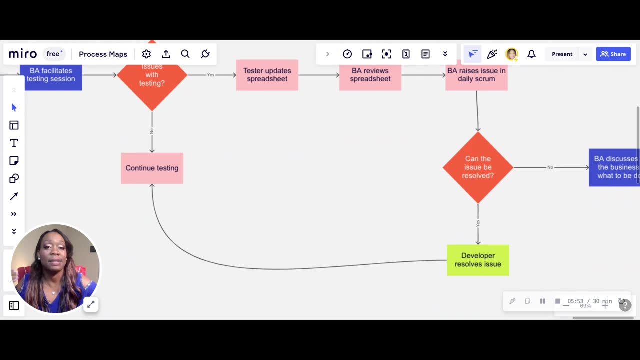 issues in the daily scrum. the expectation would be that they would start working on that immediately. Once they raise this issue in the daily scrum, the technical team would have to evaluate the bug to see if it's something that they can fix right away or if they need a workaround or what can be done. 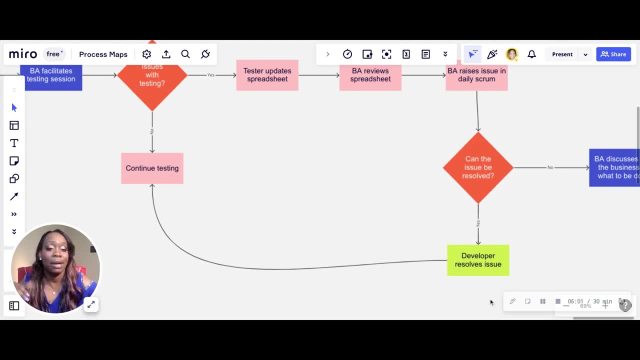 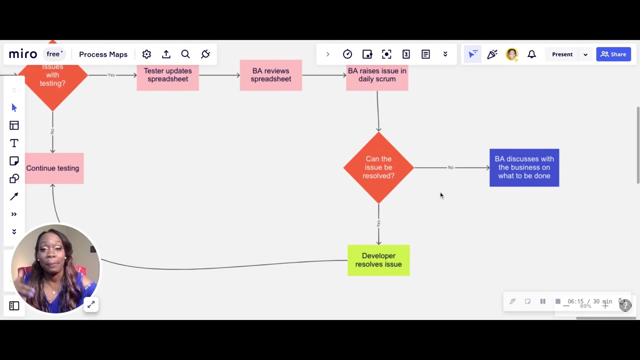 about it. So if they can fix it, then the developer goes through and resolves the issue, makes the fix and then pushes it to the environment And then the tester can continue testing. If it cannot be fixed, then the BA would have to take it up with the business or the product owner or the project. 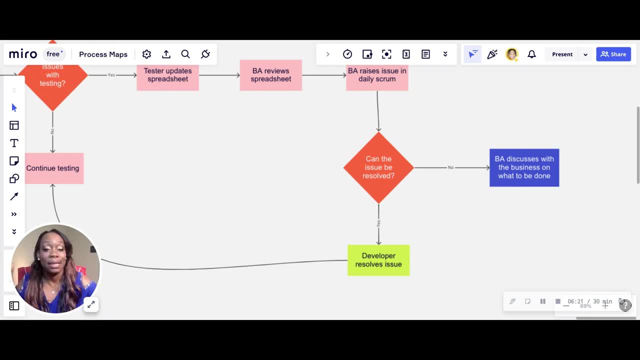 manager to say: here we have these bugs, We have evaluated them. They cannot be fixed in a short time for the release. What's the next step? right, And they'll figure that out here. And this could be a predefined process box instead of a regular box, but you get what I mean. So that is the 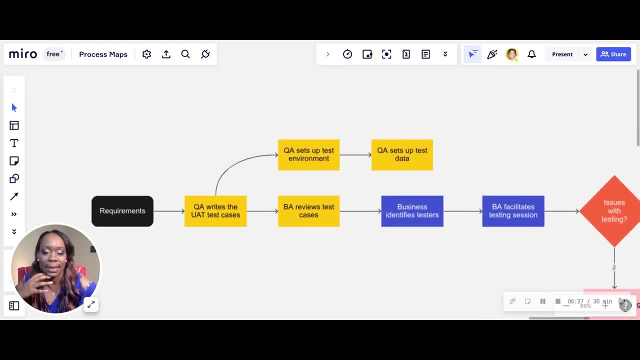 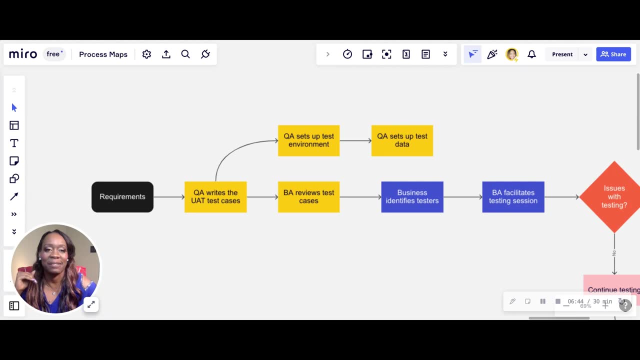 process. That is the process that they were going through for their UAT. Now this process has many holes. There are many things in this process that need to change, because if you don't make a change, you're going to end up with a lot of 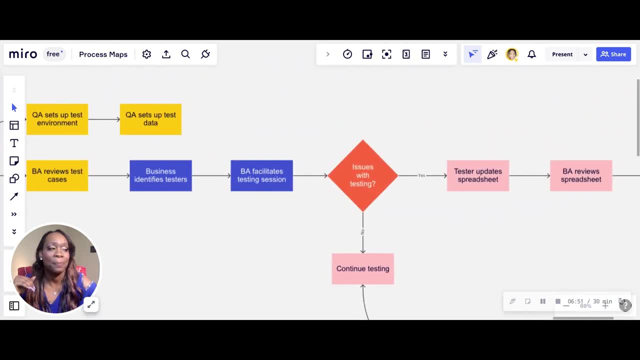 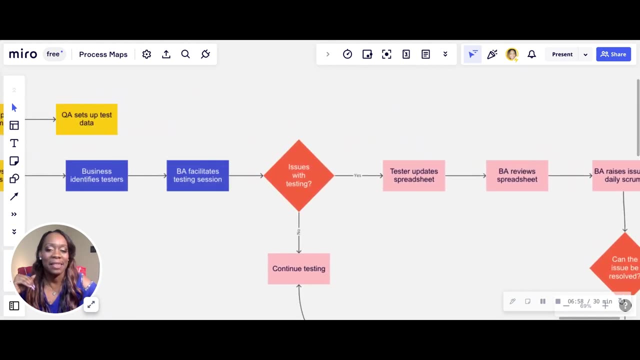 problems with this process. Does anybody identify any of the issues with this process? I wish I could hear you guys. I know you're thinking about it, but think about the first step here. right, The QA is right in the UAT test cases. So I have below here some- you know, a revamped process. 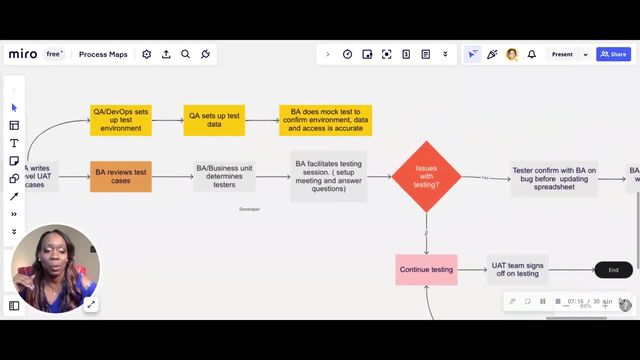 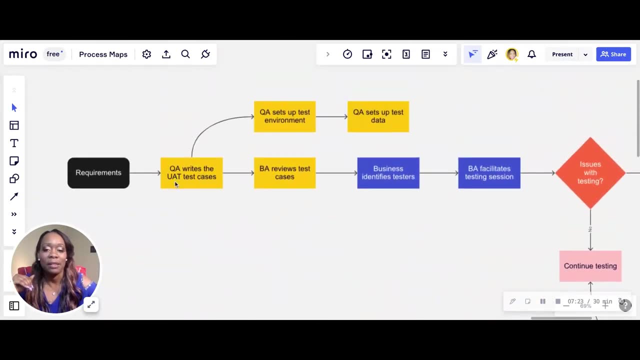 that I make suggestions as to what we could do to improve this process And I'll go through that to show you where the issues are. But just going back to this, the first issue I have here is where the QA is right in the UAT test cases Typically. 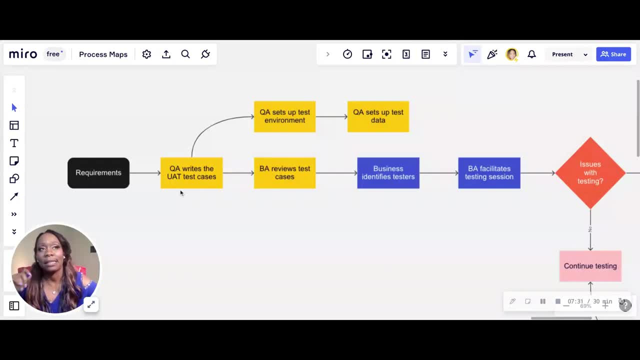 UAT test cases are written by the BA And there's a reason for that: because QA is used to doing very detailed tests. They're used to doing unit testing, They're used to doing regression testing, They're doing automated testing. So they're down in the details. They do click by click by click by click. 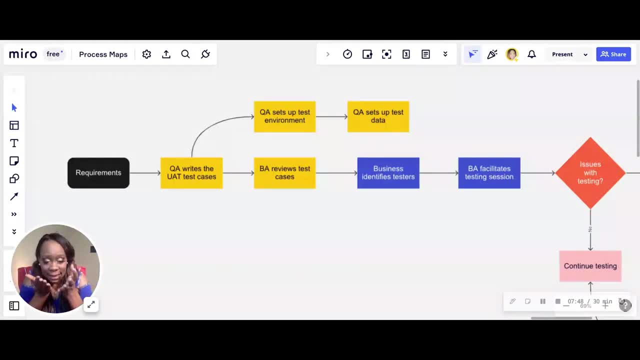 So sometimes it's very difficult for them to just come out of that scale and to give you a high level. This is what we're trying to accomplish. So because the QA comes in after you have implemented their testing to make sure the implementation is correct. 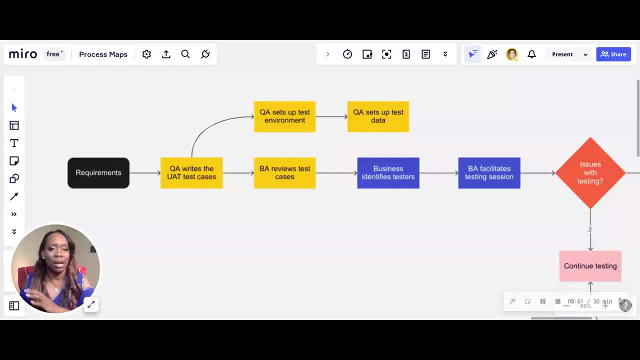 it matches the requirements. They are typically not involved too early on, So sometimes there's a disconnect between them understanding what is the actual business problem we're solving with this feature And if you can train your QA and give them up to speed as to saying. 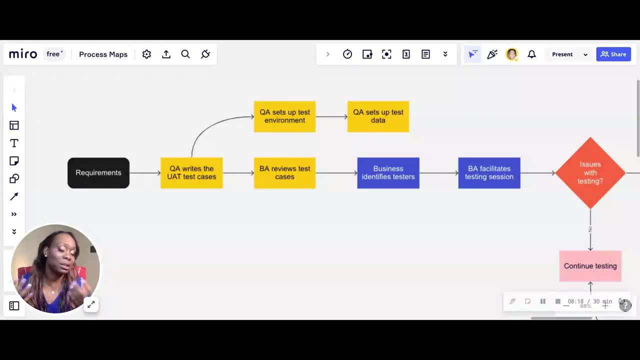 okay, what we're really trying to solve is this issue, and this is why this feature is important. then maybe we can walk them through that. Then in QA, people are pretty shocked, So maybe that will be fine, But I've just found that the level of detail in what they are writing is way too. 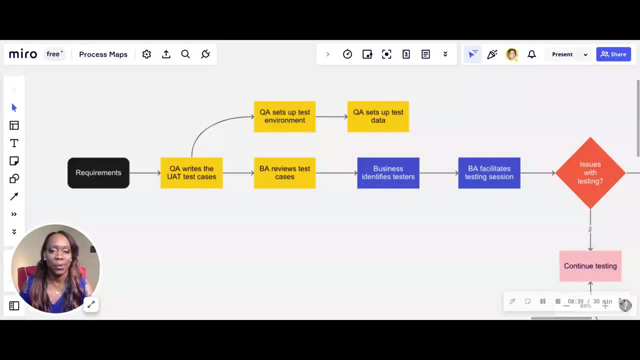 detailed for a regular tester. So that's why the BA typically writes the UAT test, since you don't need someone to say: click on this button, then create the form. Then, on the form, there's going to be these fields: Fill in the name field. fill in the address field. fill in the email field. check to make sure the email field doesn't have the correct name field. If you don't like the name field, then you don't have to. If you're going to write the name field, then you can write the address field. If you don't like the name field, fill in the email field. fill in the email field and then click to desktop the field for the other fields. 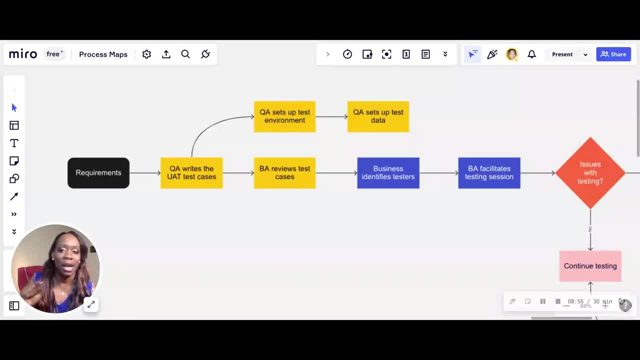 the correct uh formatting and if you make sure you get an error, the error should say this and this. they go into detail, detail, detail and that's not necessarily how you want to test, because you want to allow your testers to find bugs. so to allow them to find bug, you have to let them explore. 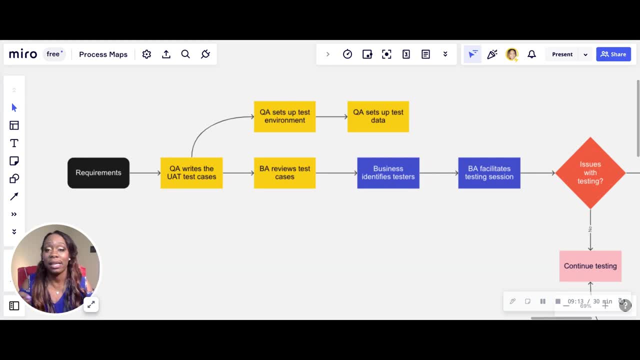 so, instead of giving them instructions that says click here, then click here, then click here and enter this value and then choose this option, you want to say something like: create an application, let them figure out how to create it, and then figure out what doesn't work. let them figure out. 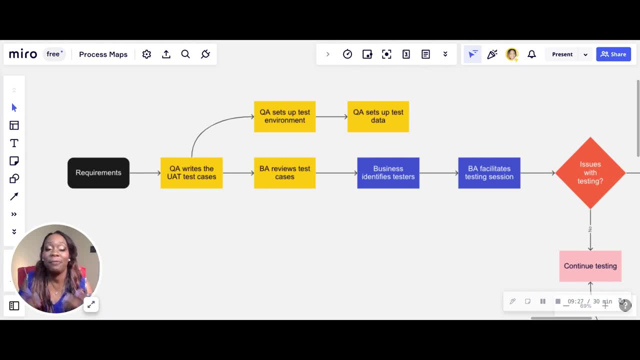 which fields don't don't feel natural for them to fill in. let them figure it out and let them tell you how it feels, because in the real world there won't be a qa on their shoulder telling them what to click on. so can they use the application without you having to give them click-by-click. 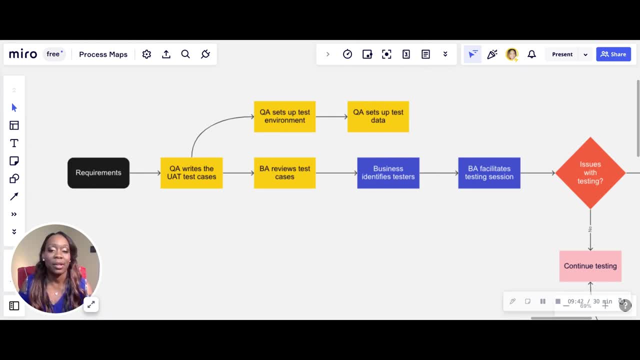 instructions. so i don't advocate that the qa writes the uat unless you really spend time coaching them and training them as to how to write high level test cases. so it's not at the level of detail that would cause the tester to be bogged down clicking. 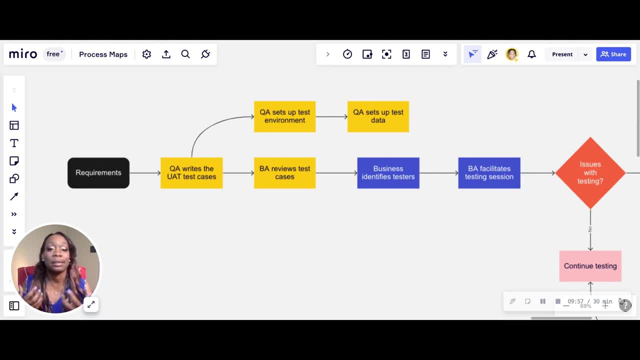 and following step-by-step instructions, as opposed to doing what they're supposed to do, which is uncover the bugs. so that's the first thing. now the qa, for sure, can set up the environment, but i find that typically the environments are being set up by a devops person, right, who makes sure? 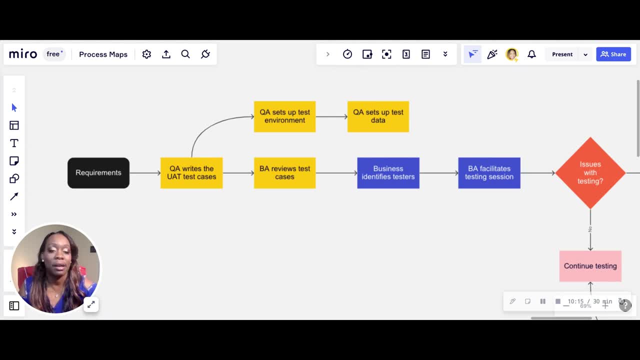 the environment is there, the apis are there, the connections are there, all of that stuff? and then the qa yes can set up the environment, and then the qa doesn't need to be set up the environment. and then the qa yes can set up the environment, and then the qa yes can set up the. 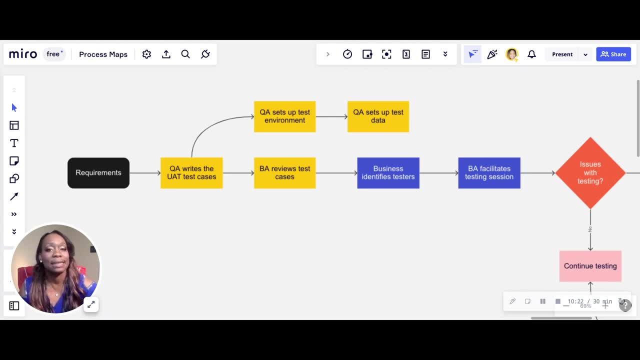 data. but sometimes you need a BA too, because if the BA writes the test cases, then they need to know where the data is coming from to fulfill those test cases and then you may have to collaborate with other teams to get the access rights and all these different things. so, yes, the 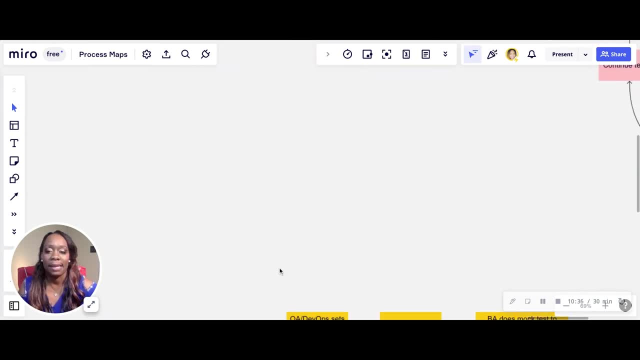 QA can help with these, but it should also be something that the BA is helping to make sure that we have all right. so this is the first thing that I noticed. then the BA reviews the test cases. so if you are able to train the QA to tell them, hey, let's keep it at a higher level, then fine when 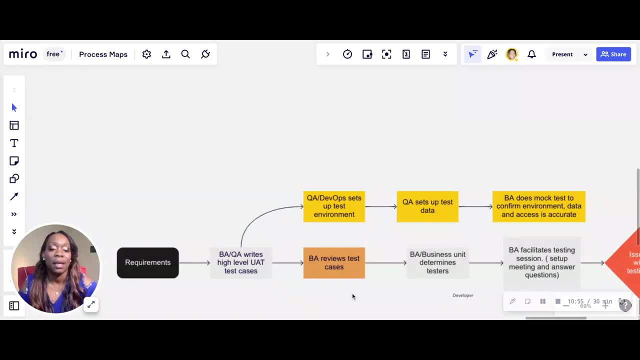 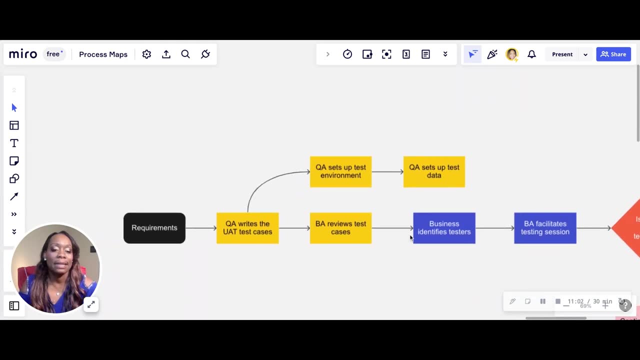 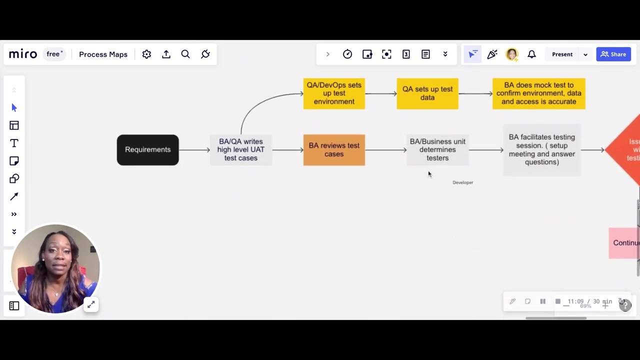 they finish it, your BA can review it, and that's great. then, once the BA reviews it- in this example, I think the business was the one identifying the testers- I would say that the business needs to also collaborate with the BA to identify the right testers, because what can happen is the business. 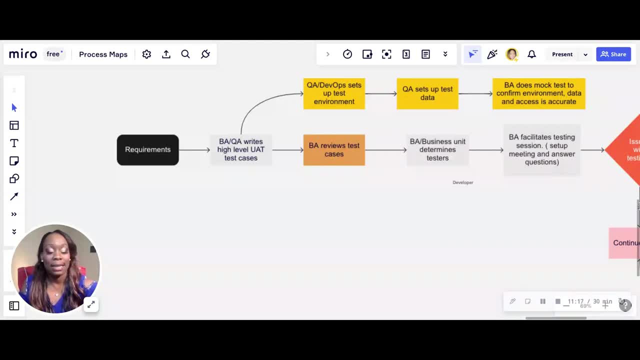 they're not as close to the technical details as you are. they know the problem they're solving for and they know what they expect the solution to be, but they're not in the weeds right. so when they choose a tester, they might be looking for the person who has the most knowledge. 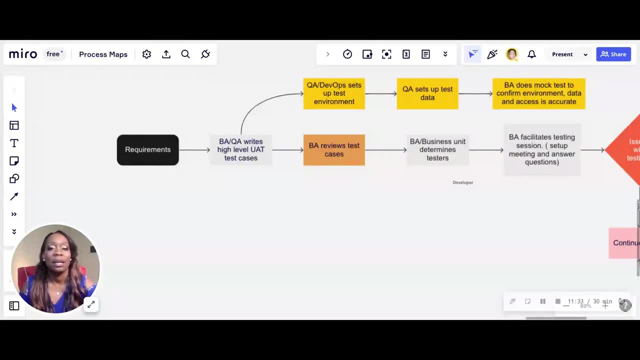 so we want to get somebody who's really knowledgeable about this so they can find out if there's any problems with it. but sometimes you want testers who don't know. so because they don't know, they're going to probably find things that the ones who know. 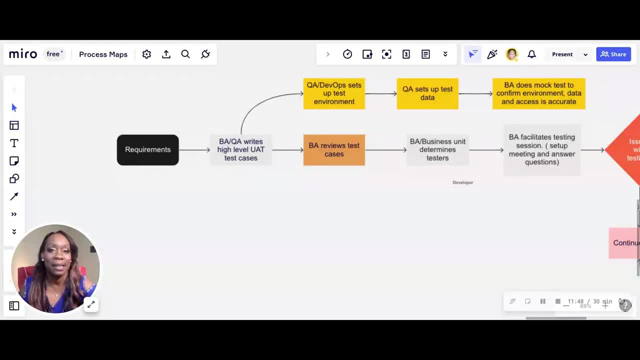 would skip over because they already know it right, so sometimes they're blinded by their expertise. so you want to collaborate with the business to get a spectrum of people: people who are very advanced, people who are in the middle, some people who are just brand new to the company. 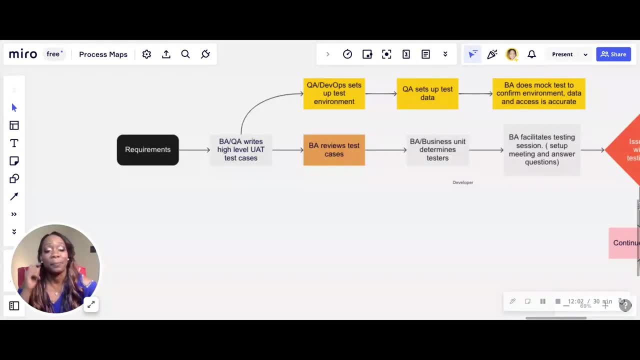 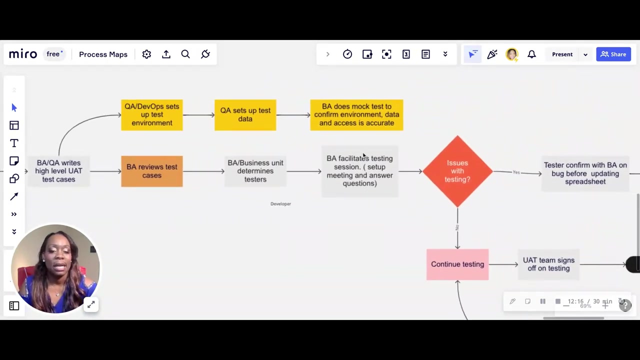 and if you can get real users, real end users, even better. so the BA would help to create that testing profile so that we get people who can help us really uncover as much bugs as possible. then the next part is that the BA facilitates testing of testing. so in the first um flowchart what they were planning on doing was have everybody test in 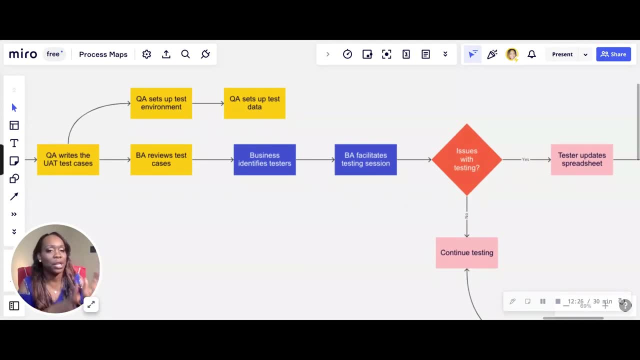 silos. so you pick your two hours and you test by yourself. you pick your two hours, you test by yourself. everybody have a different sheet. they all fill in the sheet and the ba goes through and reviews those sheets. now the project is huge. it's gonna- the uat, is gonna span over months and you 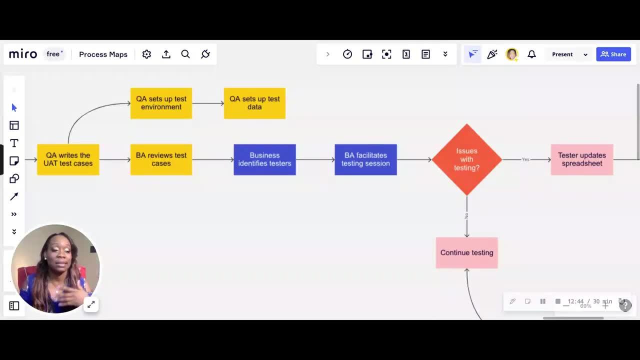 never know who's gonna come in and come out. so, as testers are being thrown in and people do their part and leave, you're going to end up with a whole lot of spreadsheets if you do it this way. and not only that, but everybody's testing in their own little world. it's connected. from the rest what? 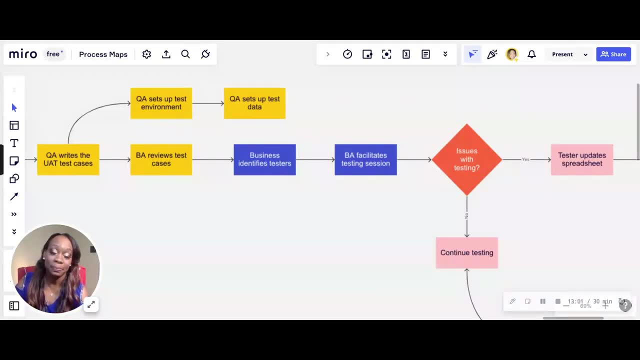 they had planned to do was have a slack channel. that will be a place for them to communicate, or a teams channel, if you're using teams, and that would be how they communicate. of course there's email, but it's just so disconnected, it's so isolated. i don't like that. i like the testers to feel. 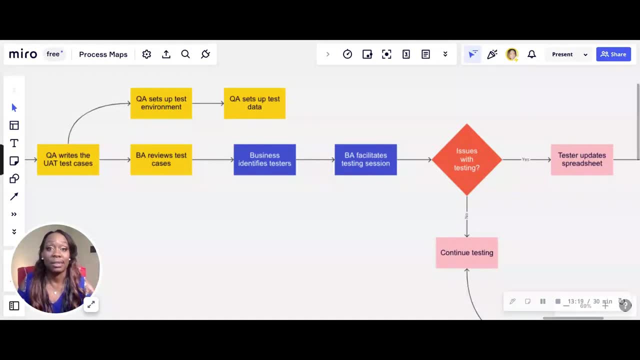 like they're a part of a team, that they are working together for some greater good for the company, and to know that they have support. so if this testing exercise is one of the biggest things that the company is looking to have done, then they have to be able to join at the same time. 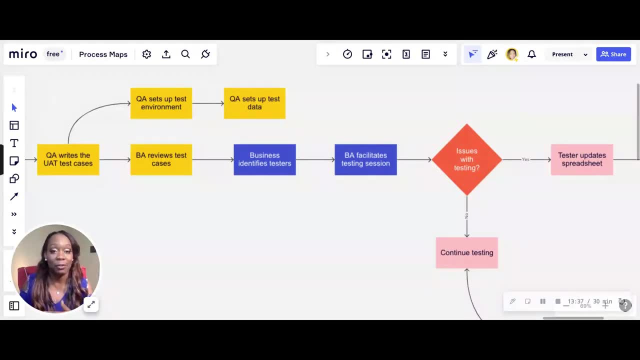 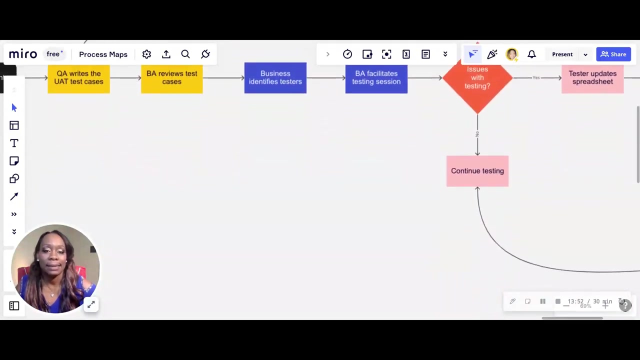 so whatever other meetings they have, they have to cancel those meetings because they're going to be focused on testing. if it's that important to the organization, then they have to make time right, there is no other um way around it. they have to make time. so i don't suggest that you have separate, isolated testing happening in silo. 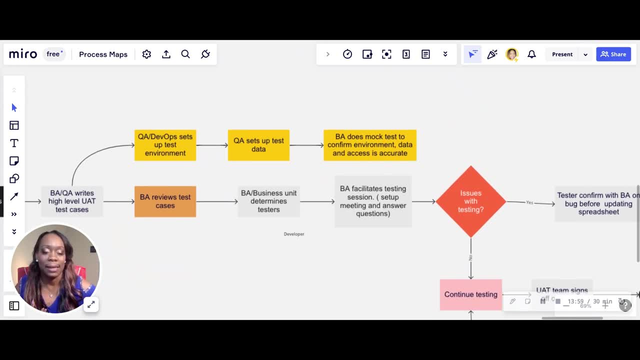 so this testing session? the way i would want it to be done is that you have the times on the calendar blocked for everybody who's going to be testing. so we're all in the same meeting and you, as a facilitator, join the meeting. you introduce them to the test. here's what we're going. 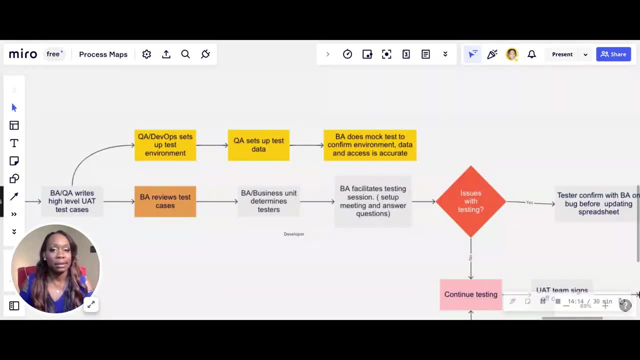 to test. here's what we're able to accomplish in today's session. here's the file that you're going to be adding your um, your bugs, to. here's how you use it. here's some: this tab does this, this tab doesn't do that- all the things that they need to know to be an effective tester you're going to tell them. 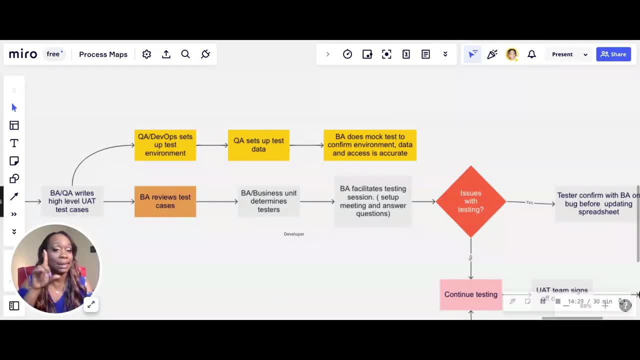 and it's one file. it's one file, right? if you want to keep backups of it, just in case somebody you know changes something, fine, you can keep a backup. but they're all looking at the same file. the file has the test cases on probably a different tab and it has this one bug tracking. 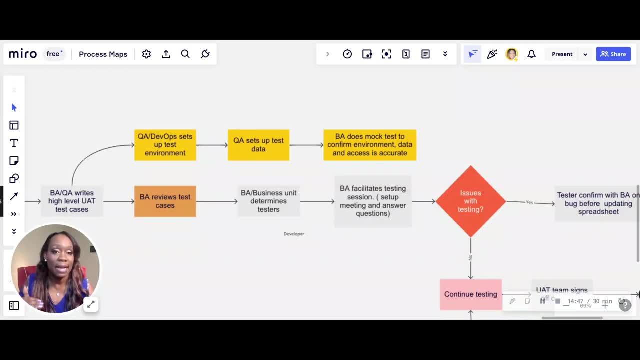 list that has all the bugs that they've found from the different different tests. right, because you want to provide support and you want everybody to be there, and the best part of this is if one person has an issue- they found a bug- i would encourage them to come, you know, if they're. 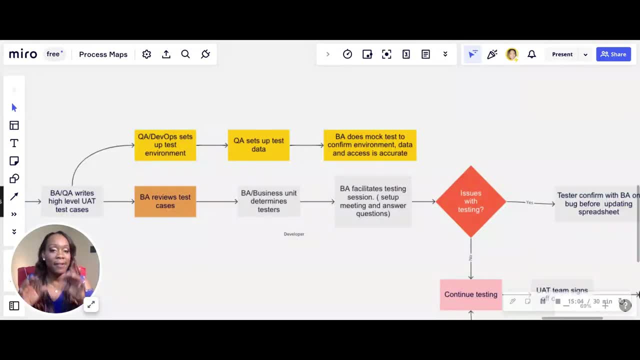 in the meeting, everybody's on mute doing their test by themselves. if anybody has an issue, they raise their hand or they jump off mute. say: hey, carolise, i found this bug. i was doing this is where i was. is this something you want me to log? it's a bug. they log it. i know the other persons on the call who heard that conversation. 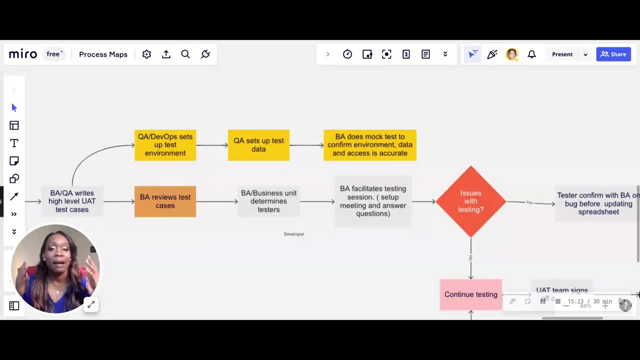 if they have the same issue, they know it's already been logged. it avoids you having duplicate issues. it avoids you having the same thing being reported in different ways. for example, let's say that there's a performance issue with the system that you're trying to test and because of that, somebody 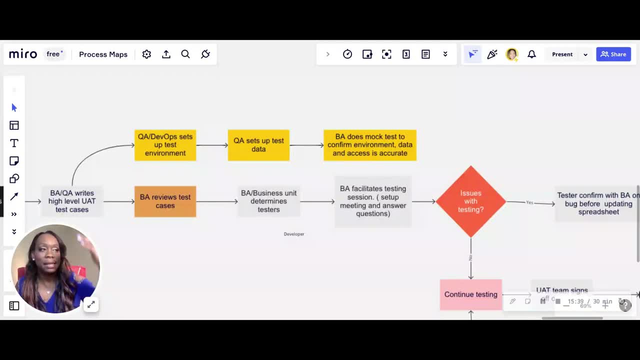 may be clicking on something it's loading, taking a long time to load. somebody else is on test eight, let's say further down. they click on something else. it's taking a long time. somebody else have is on test three and they have the same issue. and then they each might if they're doing it. 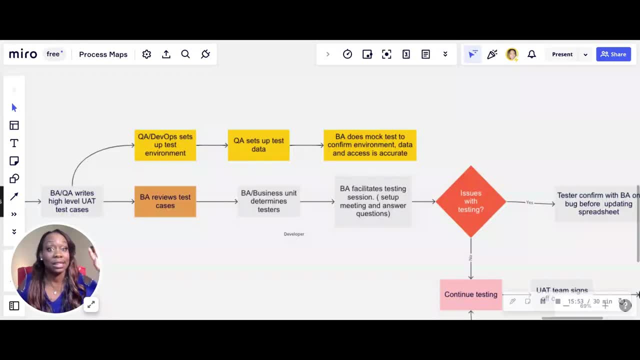 by themselves. they think it's three separate issues on, based on the screen that they're on, but because they're going to be in the meeting, one person's going to say, hey, i'm on the screen and this button is taking long to to open the next form and the other person can jump in and say, yeah, 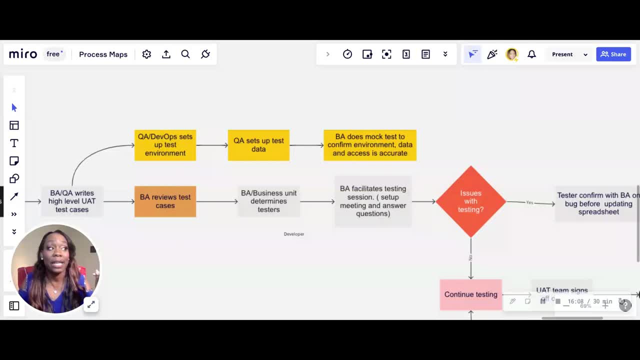 me too, and this me too, i mean. next thing, you know you realize it's a system-wide issue. on performance, there's a problem. the system is down. now you log it as one bug as opposed to five different bugs or 16 if you have 16 people in the room, because if you have them testing separately in their own little worlds, 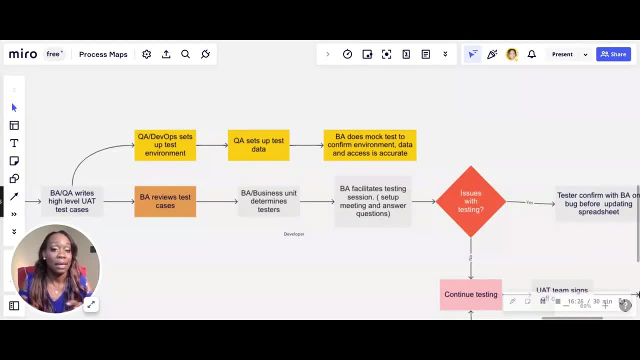 they would never benefit from that, or they could. they could probably send a teams message and say: hey, it's slow, isn't slow for anybody else, and that might help. but you may not know if they're willing to do that, because they might just be thinking: hey, i'm testing. 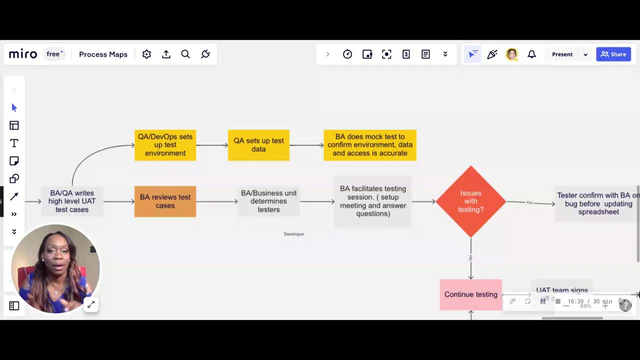 whatever i find, i'm just going to log it and i'm moving on. not everybody's going to jump on and ask if everybody else is having the same issue, do you? so what i mean so by you being there, by being a meeting where they're all a part of, and they could be on mute and doing their test, come off. 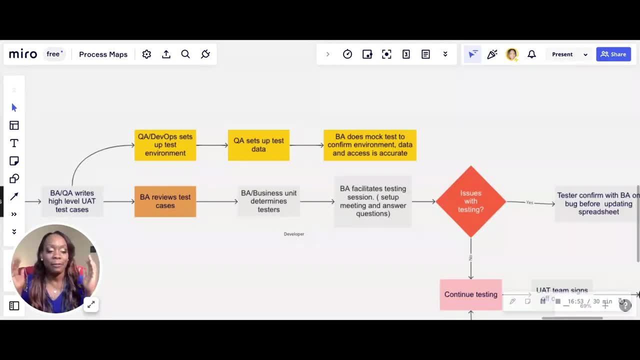 mute. ask a question. go back on me. do their test. you get them to focus on what they need to focus on. they know they're in a part of a team, they know that this is important to the company and they are more likely to focus on that at that time because everybody else is focusing on it. i think that's. 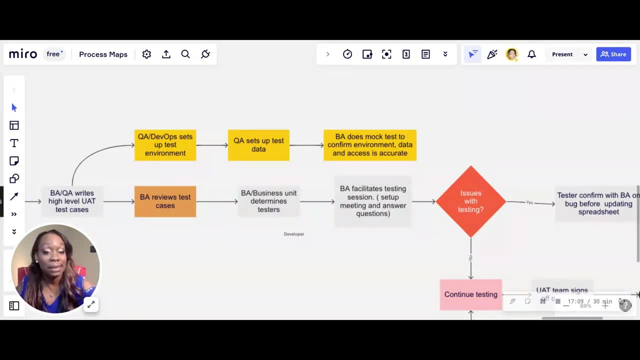 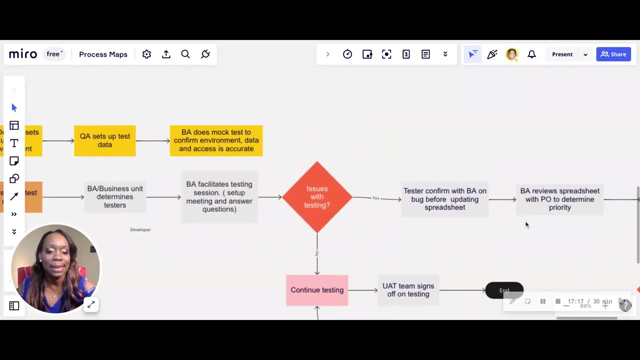 the better way to do a virtual um uat. if you can do it physically, where they're in a physical room and they have no other distraction, even better. so now, when they find a bug, like we said, it's one sheet and they're only trying to log the bug once, so they don't just randomly go add things to the. 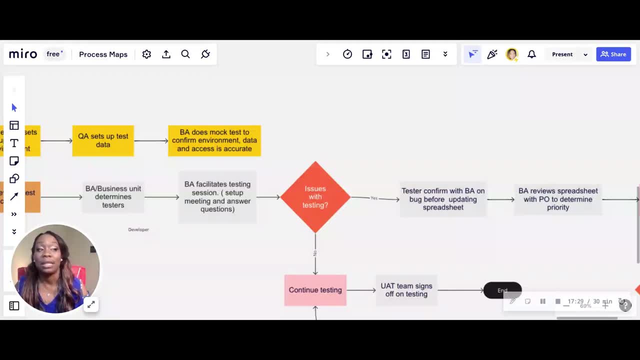 sheet, because you're going to get noise, you're going to get a bunch of stuff that don't need to be there, right? so every time they're going to log a bug, they're going to confirm with you and you're going to say: yes, this is a bug, go ahead and do it. 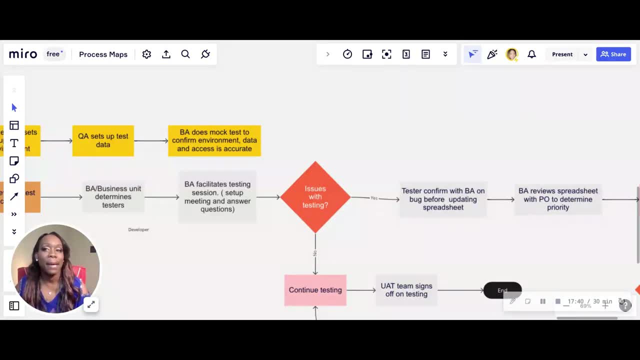 it might seem like it slows down the process, but it's better for them to confirm before they add it to the sheet than to have a bunch of noise that you're going to have to wade through anyway. so i've had in even the largest uat. it's still not too distracting for them to come off and say here's. 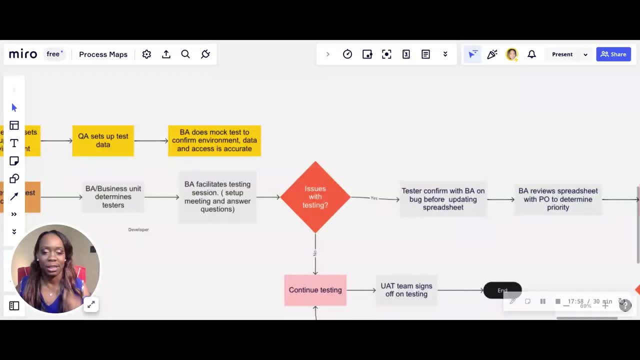 my issue. should i log it? yeah, let's log it. capture your screenshot or do a little video of what you got and that's it. it even helps because other people can hear the issue and don't log in again. so i think it's a better way to do it than having everybody adding to the sheet. the sheet is going to. 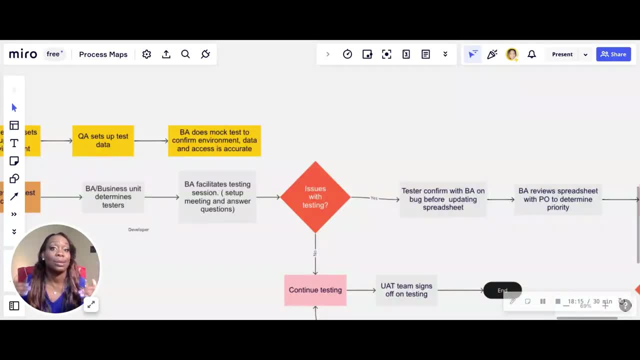 become unmanageable very quickly and you're going to spend hours and hours wading through all of this noise trying to get to the real bugs, because some of them could be, because one thing happened, other things triggered, and now they're putting all of these triggers on there, when the real source 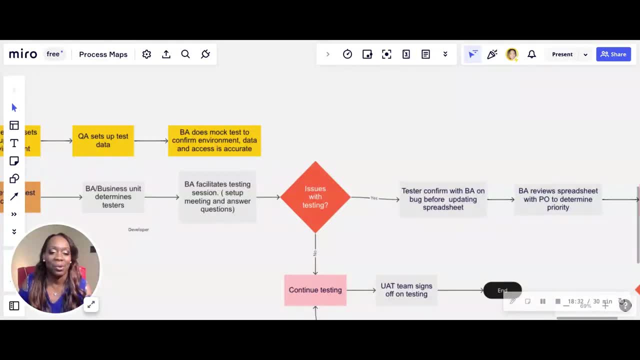 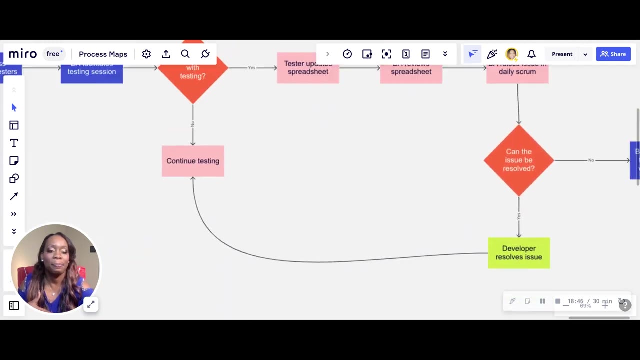 is it just one bug, and you could avoid that by just telling them and they would know what- to log the bug, because they got your approval to log the bug. the next part of it, based on the old way, was that the ba would take it to the daily scrum. so my point on that, or the way i feel about that, is: 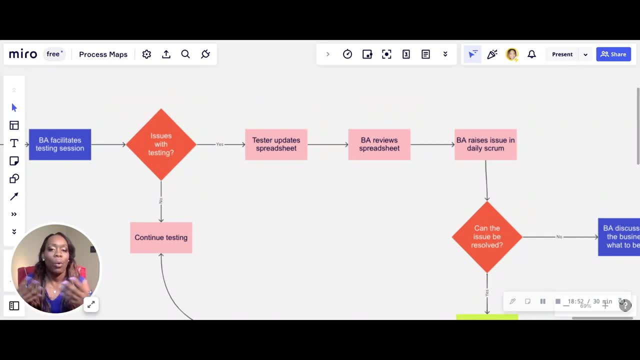 the ba should not be taking every single thing to daily scrum. what if you have 16 people testing and you have 105 issues that day? you're gonna take 105 issues to the daily scrum. that's not gonna work right. so it's. it sounds good on paper. it doesn't work in practice. 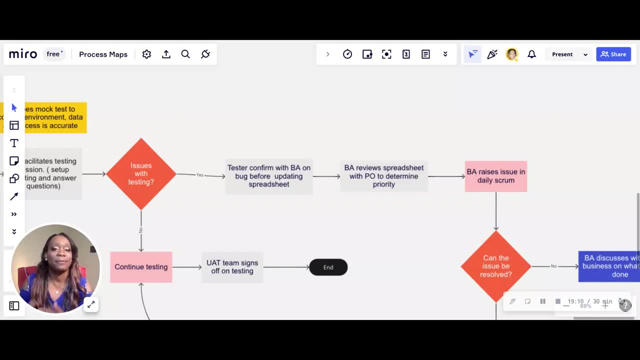 when you have these bugs. the next step is for the peel to give you the priority of the bugs. which ones are critical? which ones do we need to fix right now, before we go to retest, and has to be in the release. somebody has to make that decision because you'll have a lot of bugs depending on. 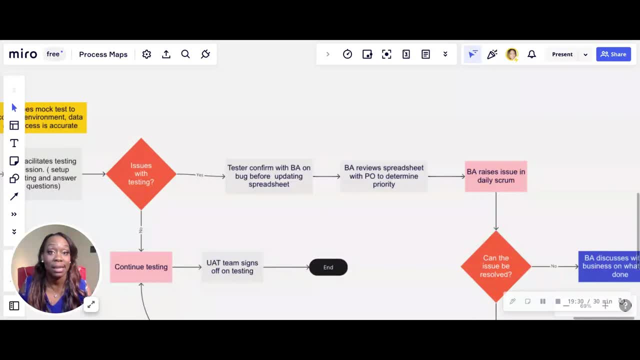 your system. you can have a lot of bugs. i've seen sheets of 500 bugs, a thousand bugs. what are you going to do with that? the regression sprint can't handle that level of bugs. i don't know how big your team is, but that's a lot of bugs. so what you need to do is, in my opinion, 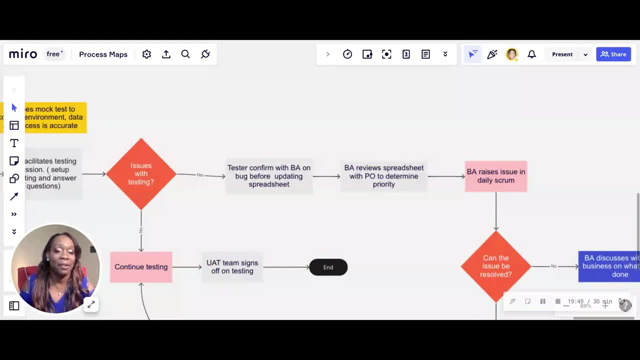 the day that you do the test. the very same day you should have a po review of that spreadsheet, and i don't want to wait till the next day because i don't remember all the details and it's you know i things get muddy. so if you can do it the very same day, when it's fresh in your mind, that would. 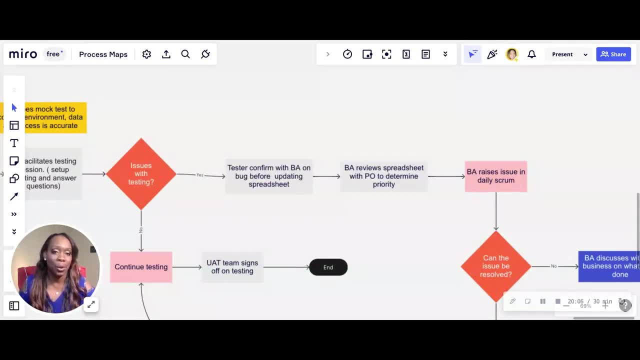 be awesome, and what you're going to do is you're going to ask the po to give a priority as to what is critical and critical and you can look at the fundamental things. right now, the people who have the most critical, who have the most critical, are critical urgent. 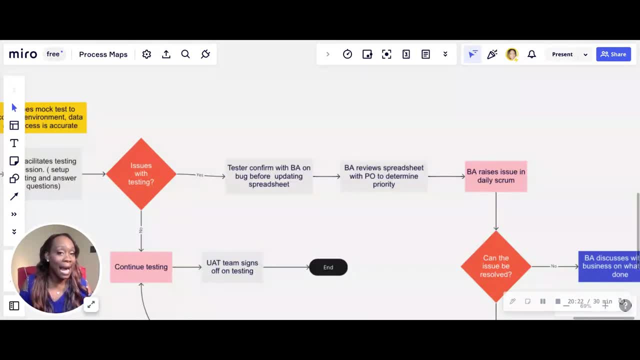 our original critical could be the same thing: critical: high, medium and low. and then you'd say: are we agreeing that whatever is critical has to be fixed before the release? yes, we agree. whatever is high, it may or may not have to fix medium and lows, definitely can some of these. 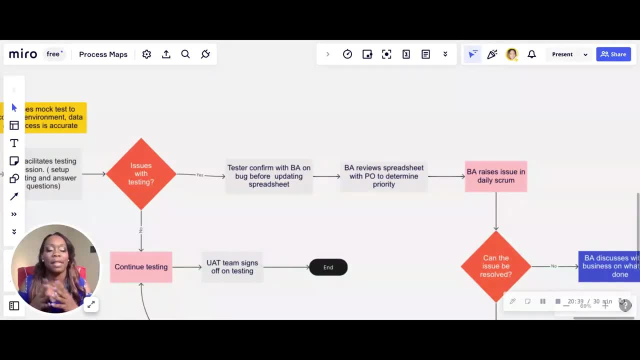 things can be, we can wait. but sometimes you can fix the medium and laws because there are quick fixes and that's what the PA takes to the daily scrum. so you take these issues to the daily scrum or maybe you have a separate meeting because it might be a. 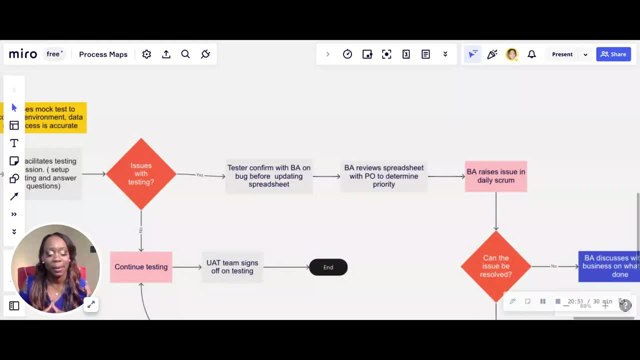 lot to go through or you might not be able to finish it in the 15-minute scrum. so you mentioned it that you have some bugs in the scrum meeting and you set a separate meeting to talk about that, because the scrum shouldn't be. 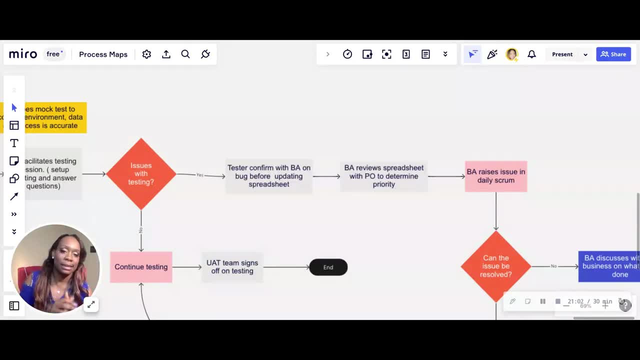 going over 15 minutes. so in their separate meeting you go through the list and you say: these are the critical bugs that we have to resolve and that's what the attention of the team should be on. so it's not every bug needs to get their attention, but that's the main critical ones that we need to get retested for. 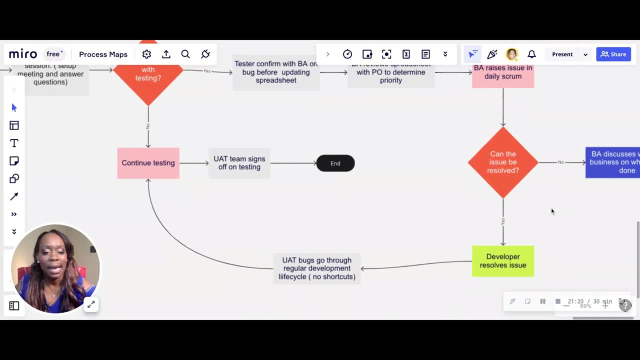 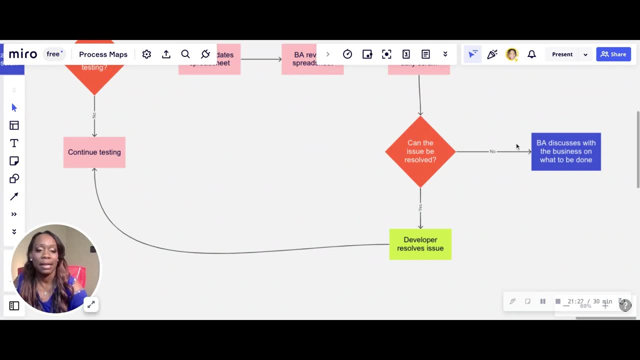 the release now. once they do that, then they go through the whole development cycle. now one thing to caution here: in the old process they would make a decision if they could fix it or not, and if they couldn't, then the business, the BA, would take it back to the business and if they could they would go ahead. 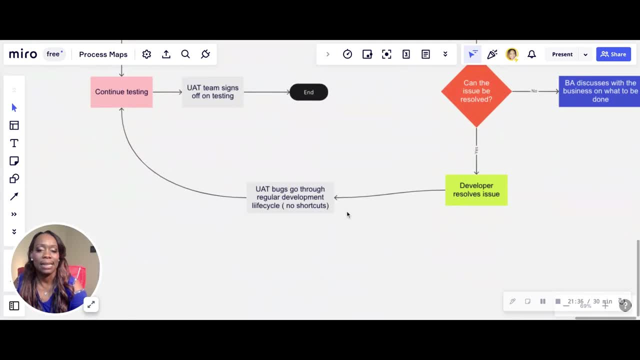 and just resolve it. but what I wanted to call out here is that they need to make sure the bug fixes go through the regular development life cycle. what I've seen in my experience is that people kind of push through the bugs because UAT is waiting to push it through. 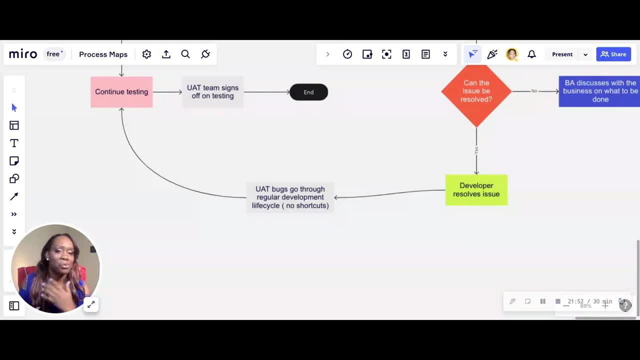 and it doesn't go through the same rigour, it doesn't go through the PR review, when all these different things, it needs to go through the regular software development life cycle and there needs to be no short cuts. you can do it faster, but it needs to be done the proper way and you can push it. 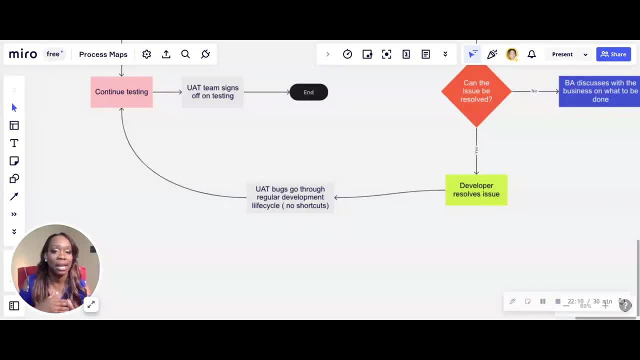 through what it needs to be done, because sometimes they push through these things fast because they're trying to get uat and it breaks other things. it wasn't tested properly and the last thing you want is to put something in front of your testers. that is a retest and it's even worse. 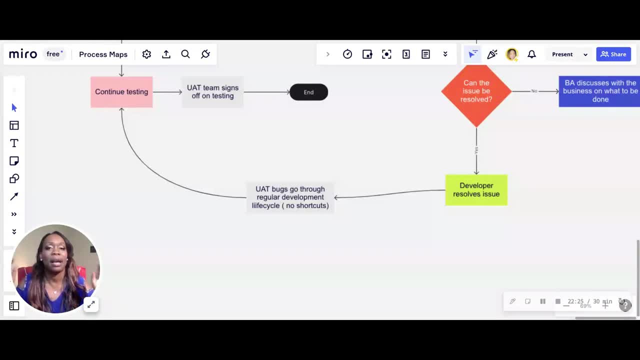 than the first test. so you don't want to put bug fixes that are not properly done and tested in front of your uat. so make sure that once they have resolved it, it goes through the proper software development life cycle. listen to wisdom. i'm telling you what i have seen in many cases. i'm giving you the, the. 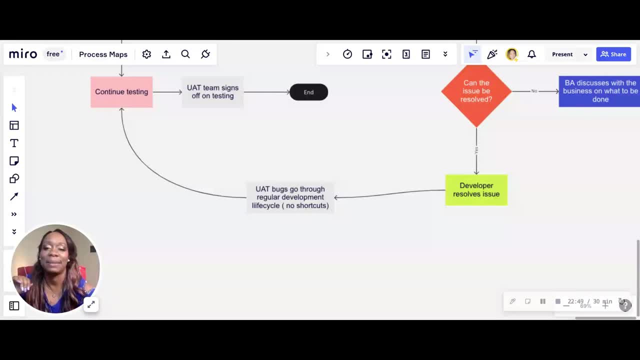 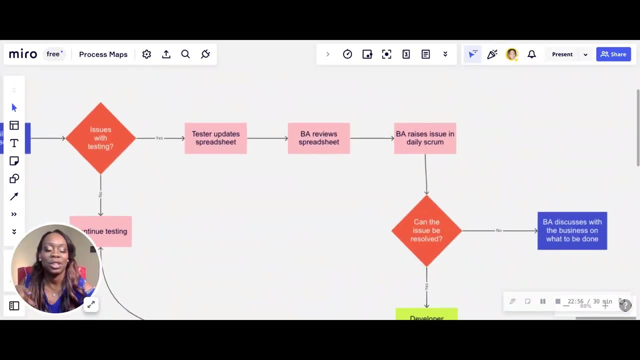 juice, giving you the secrets to success here. okay, listen to what i'm telling you now. it goes back to the test so that they retest it here, and in the first process you just keep retesting and retesting until all your test cases are, either, you know, passed or you just decide to end. 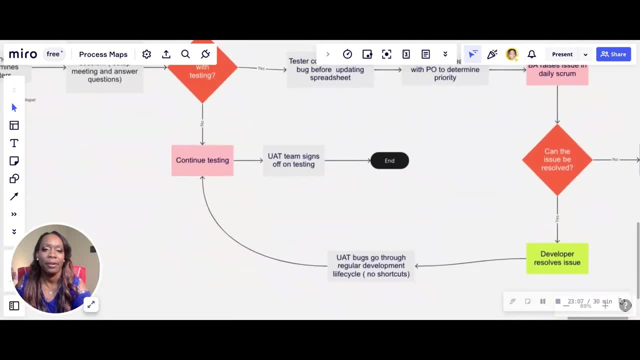 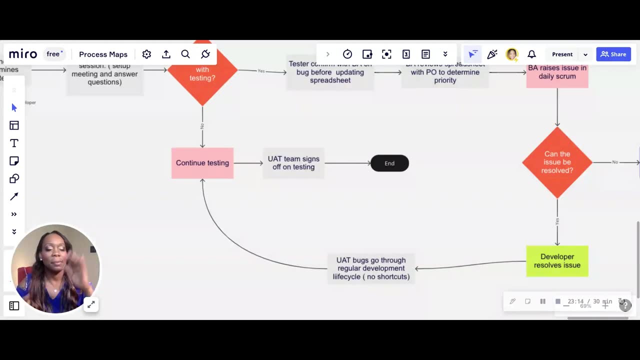 the uat. but i like to have a formal sign off where we say: these are the bugs that we uncovered in our testing effort. we list them all and these are the bugs that are high- medium. we resolved all the critical bugs. we still have some medium and some lows, and i basically go around the room and i 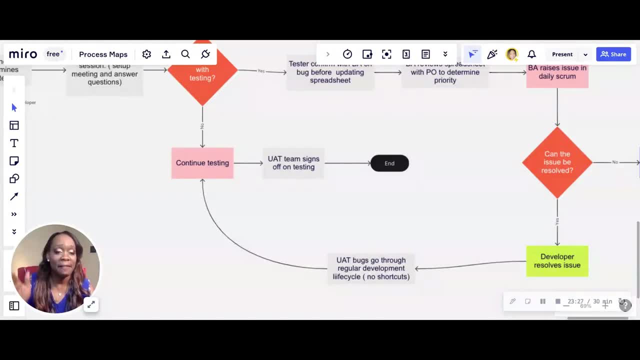 ask each of the testers whether or not they accept the features that was presented to them to test and they give their feedback and at the end of the session i asked them if they would all agree, if they would all agree with which test we are testing, that we can release this feature to our client base, given that we have these. 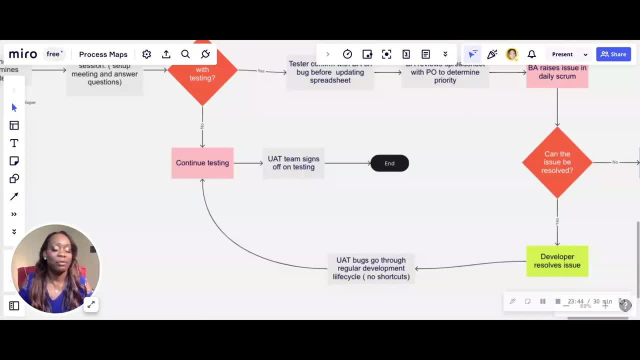 maybe low bugs that we haven't gotten to yet, but we have merely we've met the main deliverable requirement and we have fixed the critical bugs. and they would all say yes, they give a thumbs up, or they would say yes, and there's a sheet and they sign off and say yes, they agree, and that's it. because I like to take 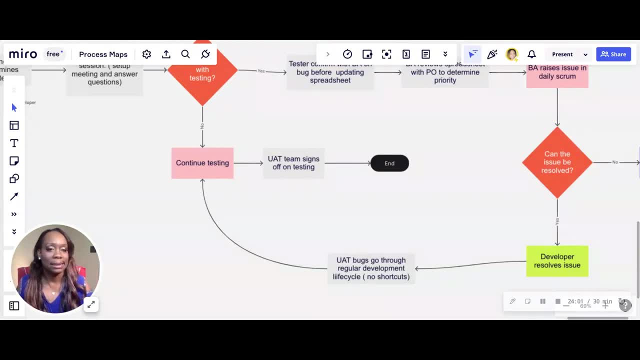 that back to the project team to say we completed this testing exercise. we had 16 testers. they went through these different features. at the end of the testing they agreed that this is acceptable for them to put for us to put in front of our customers and they felt happy with the results of the testing. 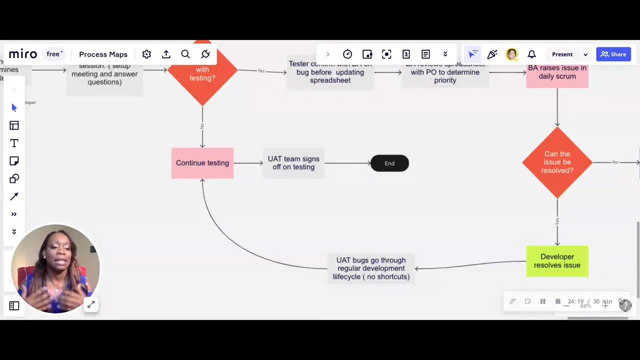 they learned how the features work because of the testing and they believe that it solves the main problem. I want to have that talking point. so when I have this formal sign-off, I feel like I put a nice punctuation point on the UAT and I get a nice close to the UAT. so 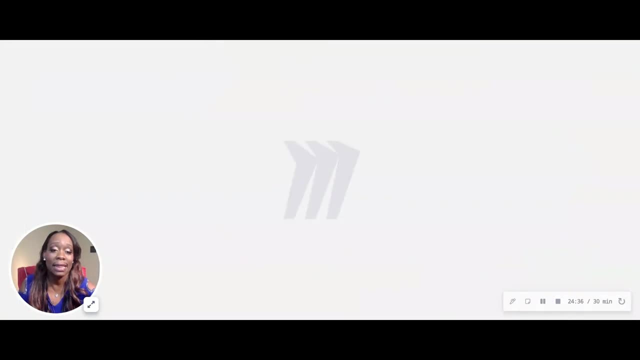 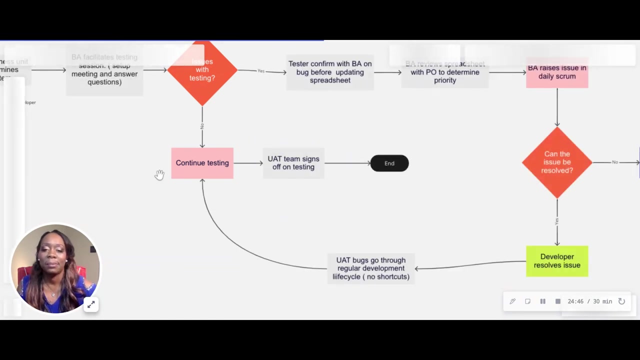 you. that is the UAT process that I think. oh, what did I do here? I went out of the board. all right, hold on y'all, it's coming back, okay. yes, so that is the UAT process that I think makes the most sense. again, everybody's doing their own. 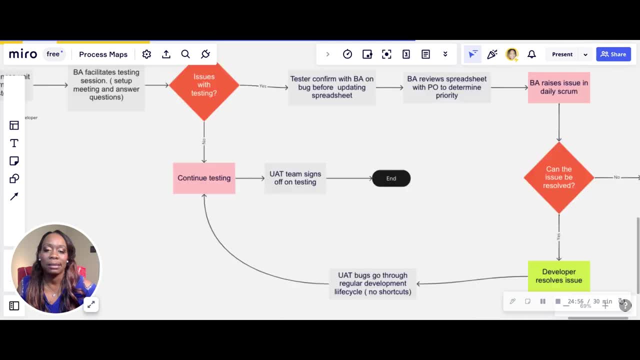 thing. so you know, it doesn't mean: this is the, you know, the be-all for UATs, but I have just found that this: this is the be-all and end-all for UATs. but I have just found that this: this is the be-all and end-all for UATs, but I have just found that this. 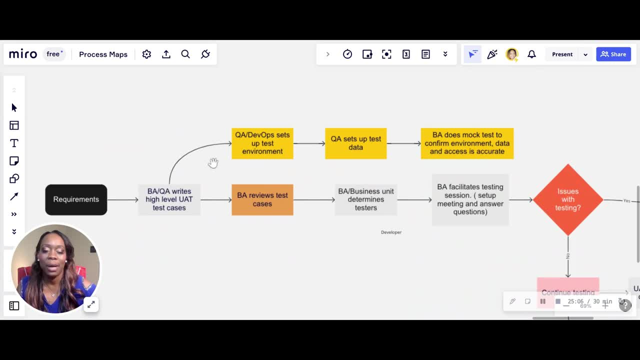 process works a lot, and also one more thing I didn't mention is when you have the QA setting up the data or even the DevOps, you, as a PA, need to run through this test, do a mock test with the UAT to make sure that everything is working.